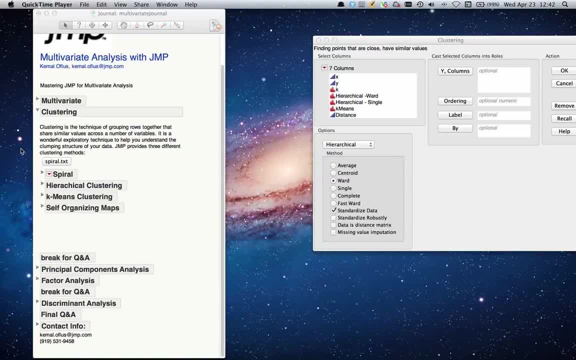 The next topic we will be talking about is clustering. Clustering is a technique of grouping rows together that share similar values across a number of variables. Imagine you have thousands of rows of data and you have 20 to 30 different variables. It will be very hard to put all your observations into one or two groups, depending on either variable 1 or variable 2 or variable 4.. 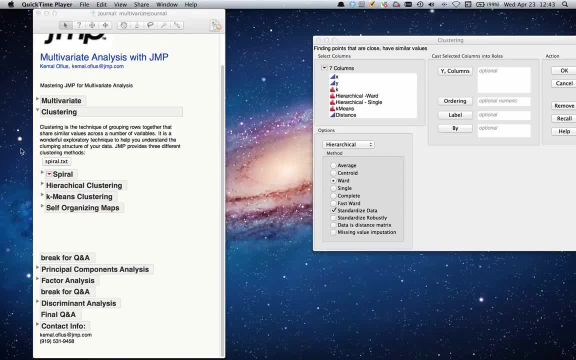 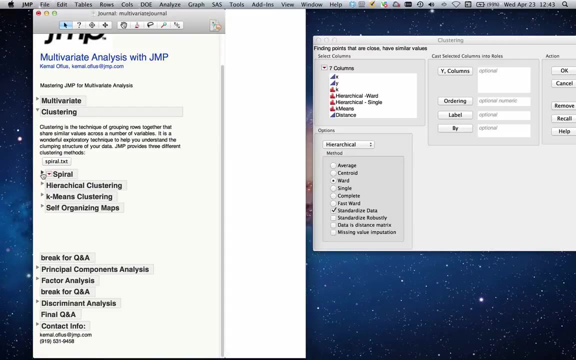 In most cases, all those variables will come into contact and give you an underlying structure. So clustering technique will allow you to find the underlying structure in your data. Let me put it into an example. This picture that we have on the screen is a picture of a spiral. 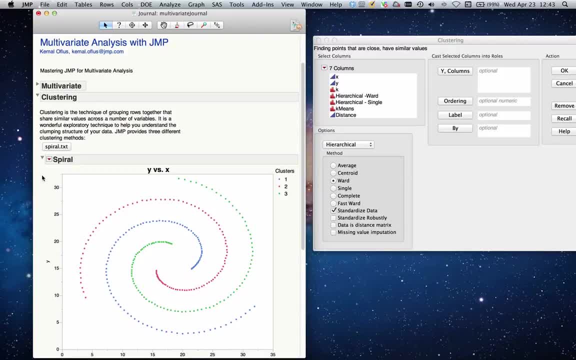 For a human eye, this is a very easy process to identify each of the lines of the spiral and put them into different groups. But if it is a human eye, it is very difficult to identify each of the lines of the spiral. But if it is a human eye, it is very difficult to identify each of the lines of the spiral. 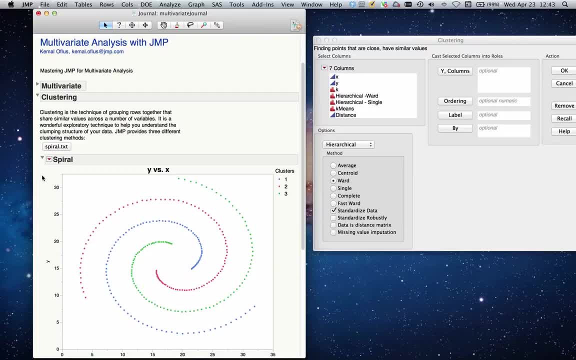 If you were to solve this problem in a computer case. In most cases, the algorithm will be able to pick up your upper half or lower half or lower left corner, lower right corner, upper right corner will allow you to be able to identify. 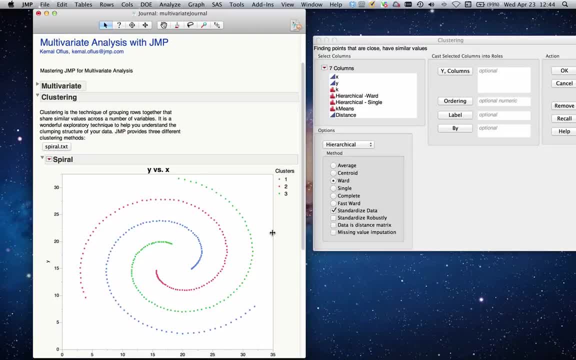 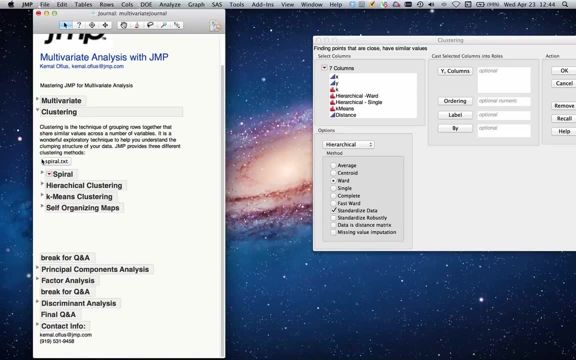 find the underlying structures on your data set with JMP And the different types of clustering methods are implemented. just to give you an idea, By using JMP you'll have access to hierarchy clustering and different versions of hierarchical clustering, as I will show you the dialog box in a minute. 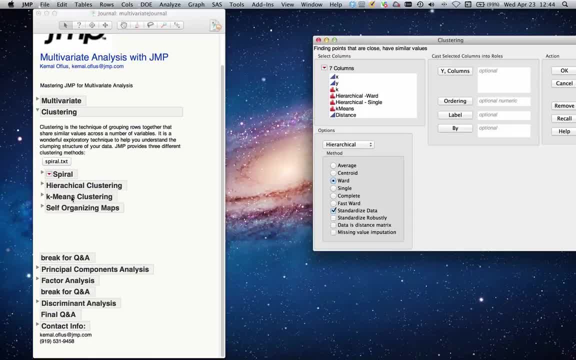 And you'll have access to k-means clustering. And also new in JMP 11 is the self-organizing maps that you will have access to use to cluster your data, And each of these clustering methods have different ways and different reasons to use it. 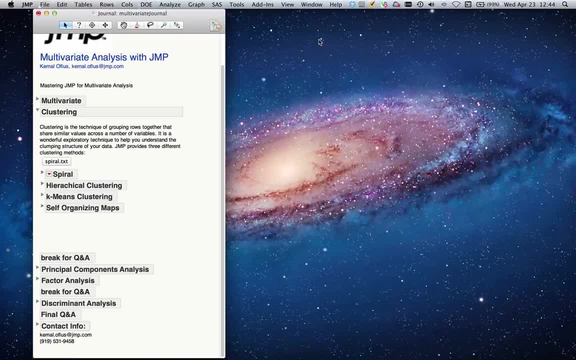 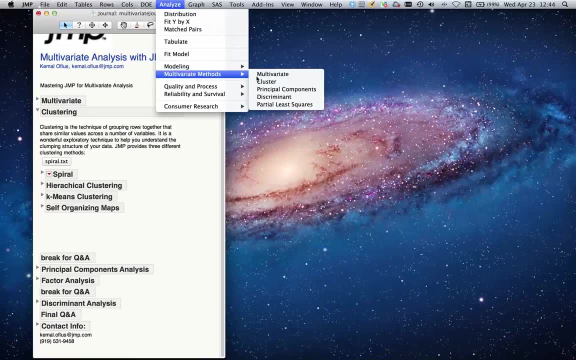 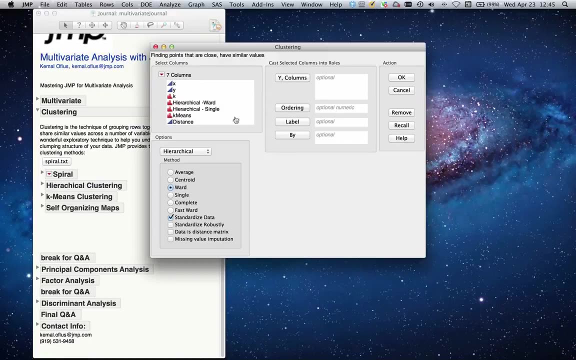 Let's go through them one at a time. First, let me show you how you will access to a cluster platform. It will be under analyze, multivariate methods and cluster Like any other dialog box in JMP. cluster dialog box is also organized in a way that you have. 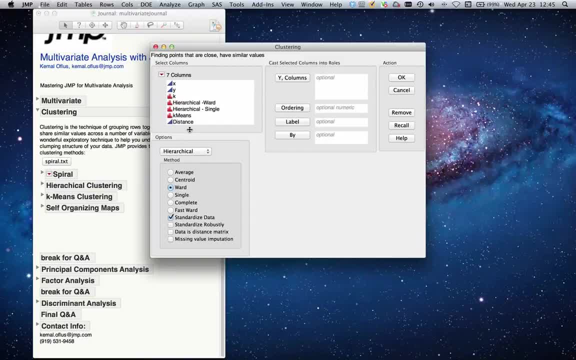 you will have a list of your columns and you will select the ones that you want to explore. In this case, I'm trying to explore my X and Y columns and I can either select them and drag it to the Y columns box or while they're selected. 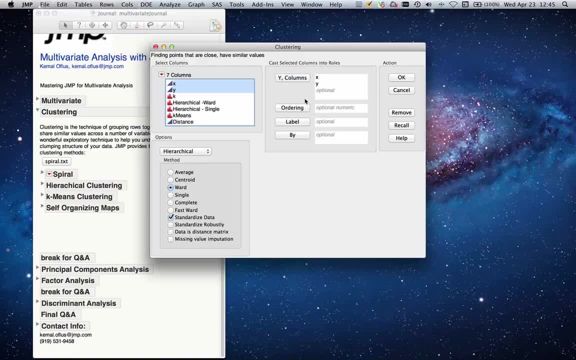 I can click on Y columns and they will populate the box for me. And then I mentioned earlier that you have access to hierarchical clustering and also k-means clustering, where self-organizing maps will be under k-means clustering. Now, before we move forward, let's talk about 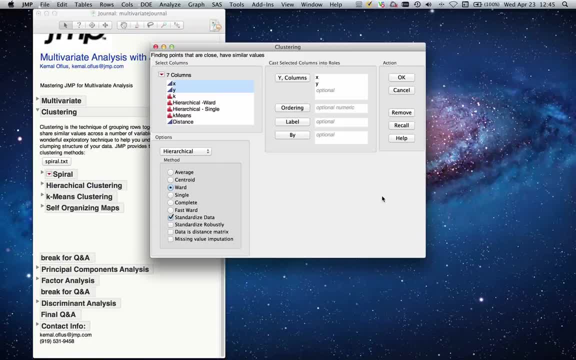 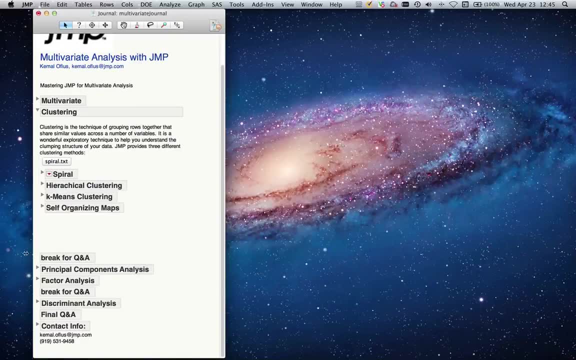 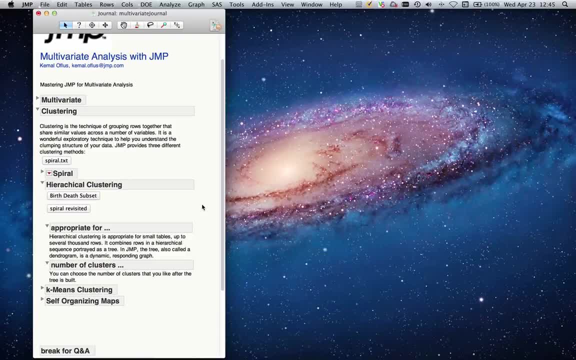 for small tables up to several thousand rows And I say and I say small tables and I said several thousand rows In the scale of data sets being analyzed, explored with the cluster methods. thousand rows kind of small data set. It combines all these rows in a hierarchical sequence. 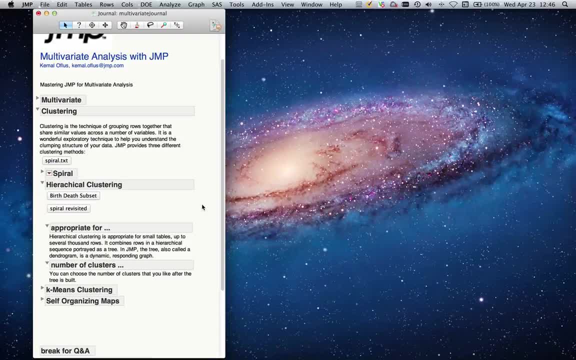 and as a form of a tree. In Jamf this tree is also called a dendrogram. So you have the tree and then you have the branches coming out of the tree. Now, another thing to keep in mind when you're building clusters is number of clusters. 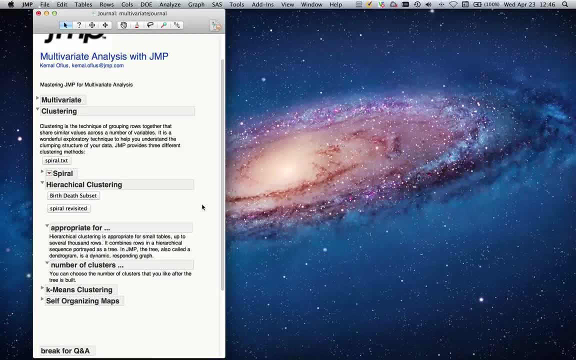 With the hierarchical clustering, you can choose number of clusters that you like after the tree is built So you can have a quick view of your tree and the dendrogram and you can decide where to cut your tree. Let's look at it as an example. 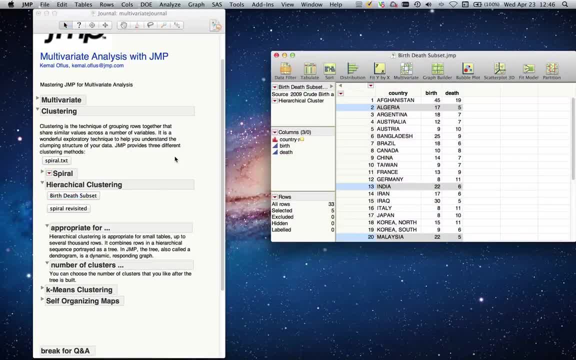 I have this data set and this is a list of about 33 countries and they have the birth and death statistics for each of these countries And I want to put them in an organism in a way. I want to put them in certain clusters. 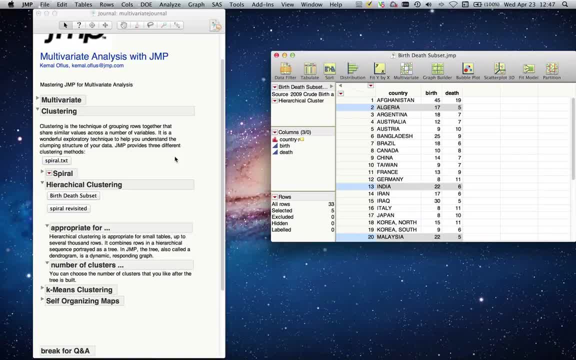 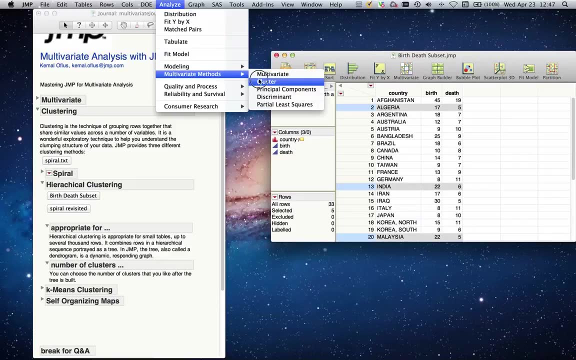 so they will have same birth and death characteristics. So, depending on where they are, it will only be depending on the birth and death rates in the country. How I would go about doing that, I would go under analyze: multivariate methods- cluster. 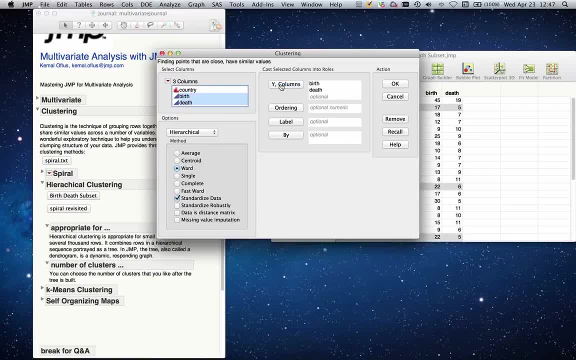 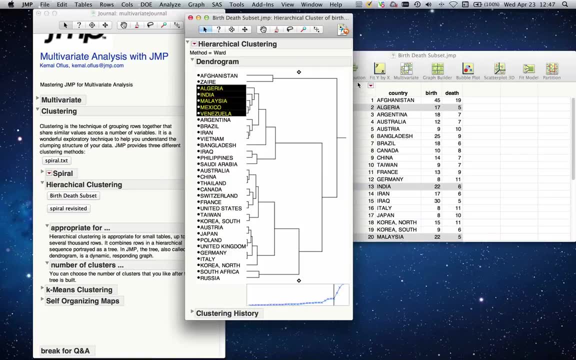 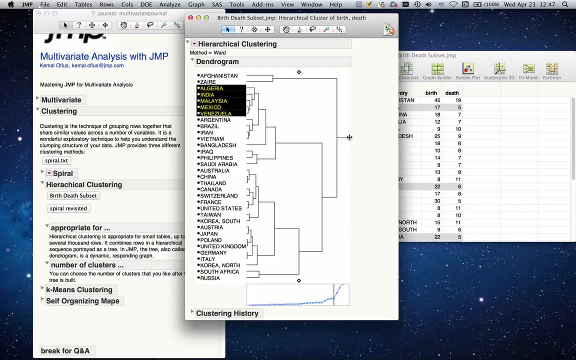 and I will select my birth and death records as my Y columns and click okay. What will happen is it will go through my data set and build this dendrogram tree for me And if you look at this, it's sort of like a sideways tree. 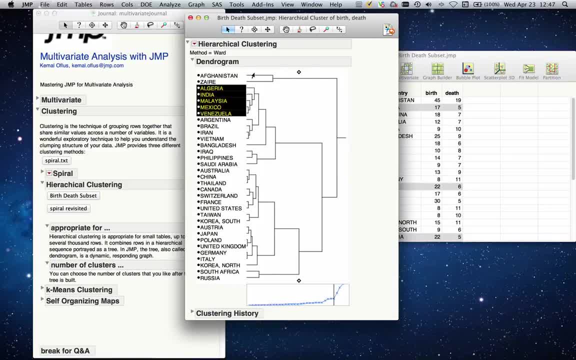 and I have my bottom trunk and it branches out and it branches out again. What this dendrogram tells me is that there is some relationship between Afghanistan and Zaire, depending on your birth and death rates, And also there's a relationship between Austria and Japan. 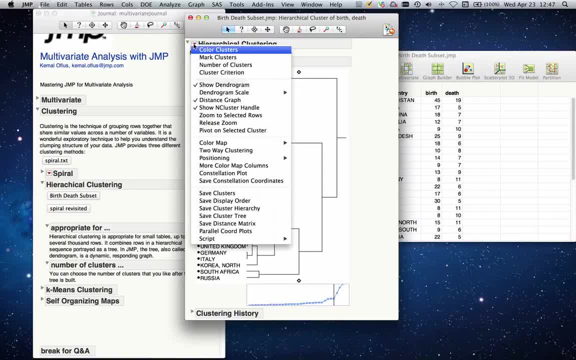 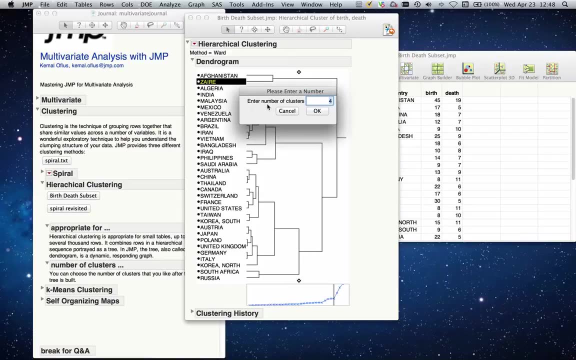 And I mentioned earlier that you can decide how many clusters that you want under this red triangle, where almost all your options are hidden, and jump In every other platform. you can decide number of clusters. you can decide how many clusters that you would like to show in this data set, and I just picked number four. it depending 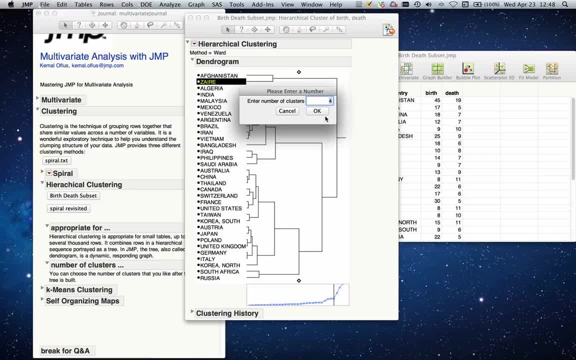 on how comfortable or how much differentiation do you want to make in your data set. you can make this tree as thin or as thick as possible, so let's stick with four. and what will happen is I have the diamond mark saying that I have four trees- one, two, three. I have four clusters- one, two, three and four- and 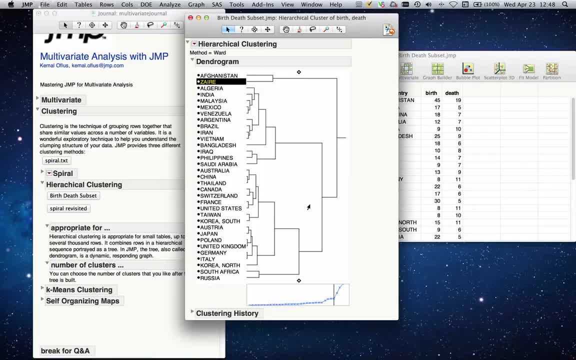 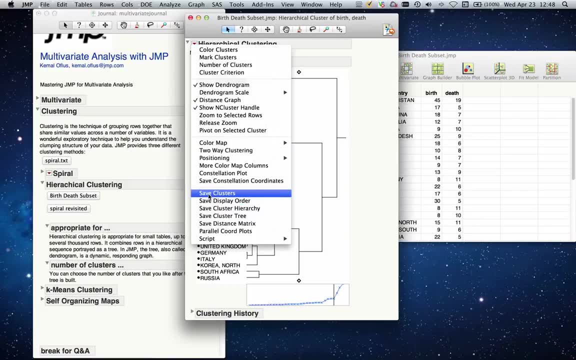 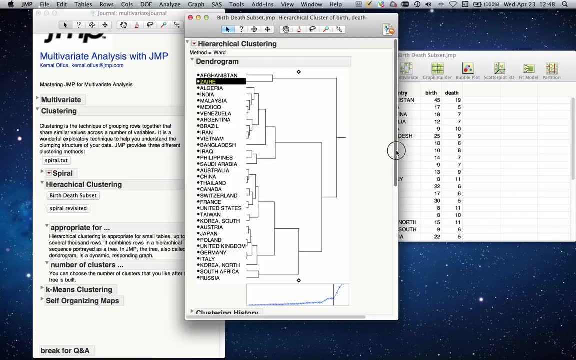 each of these clusters have its own character characteristics. and how do how do I use this clusters? what I can do is under again with triangle. I can save these clusters. but before we go to clusters, another way of looking at this tree is a constellation plot. constellation plot is similar to a 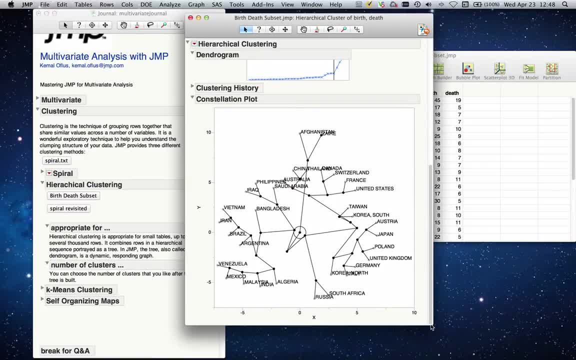 network diagram that you will find some other platforms. you probably know these are called the network diagrams. you probably know these are the Southern Facebook or some other type of networking, And here you can also see visually Afghanistan and Zyra on one branch of a tree, or Venezuela. 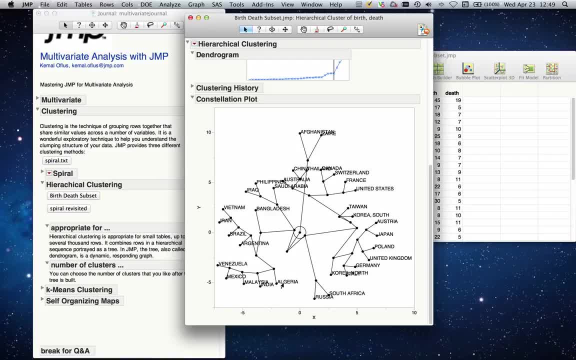 Mexico, Malaysia, India and Algeria. another branch of tree. This will be very helpful to identify if you have a lot of different variables. so you can bring it down to a spatial view. so you can identify if there is an underlying structure in your data. Another way to use it: I can come back and save. 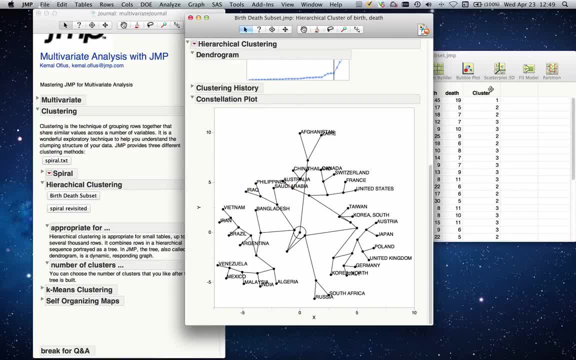 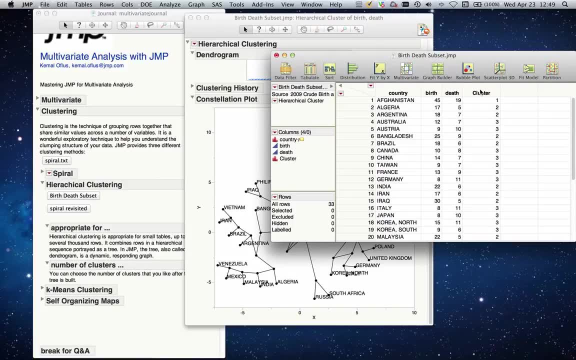 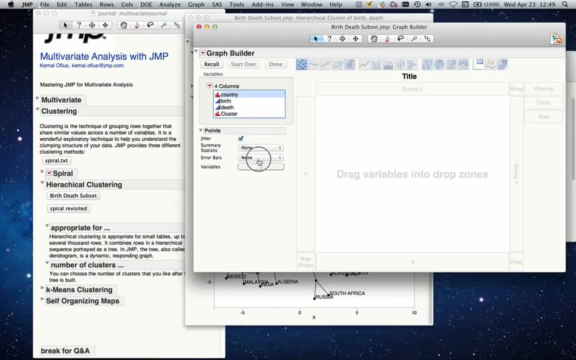 my clusters on my data set, and Jamf will create a new column on my data set, as you see here, and label it as cluster. A great way of looking at this data would be: I can go to my graph builder Under graph builder if I drag my country into. 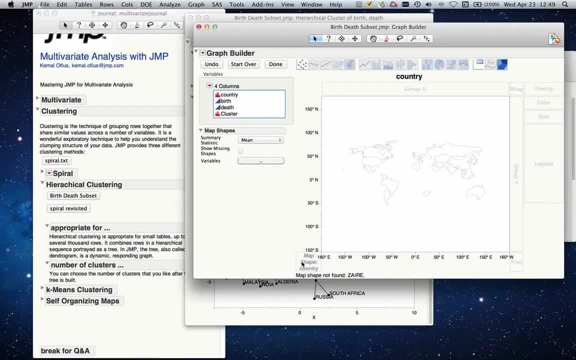 my map shape. Jamf will recognize. this is a geographical data that I'm looking at and if I want to take this data set and color it with my clusters and I can see the correlations visually, I'll go back to my data set. I want to make sure that I represent the whole earth and I 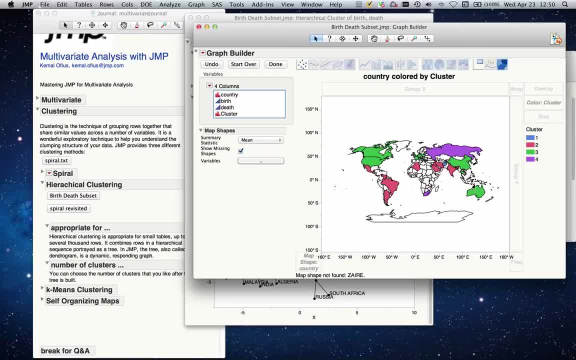 can see where Canada, United States, Australia and most of the Europe, Western world and China has similar birth and death statistics, whereas Russia and South Africa have different underlying structure, and I can see most of South American countries and tropical countries have similar birth and death that rates as well, And I can when I'm done with this, I 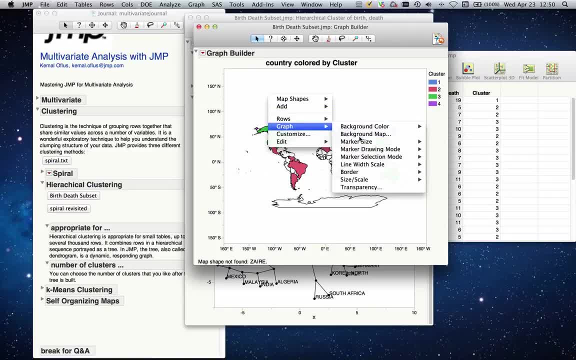 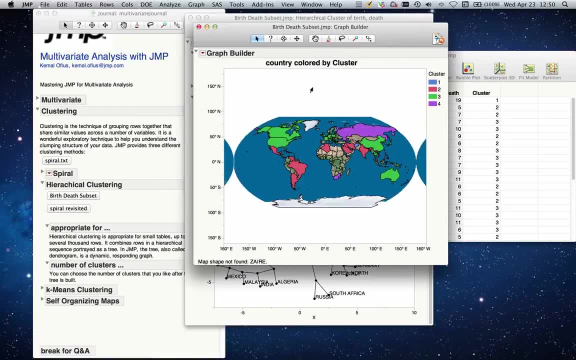 can save this, or I can modify my background map to look prettier. I can say: show me just a simple earth. This will be a great way of representing your data and once I'm happy with it, I can use my selection button copy and paste. 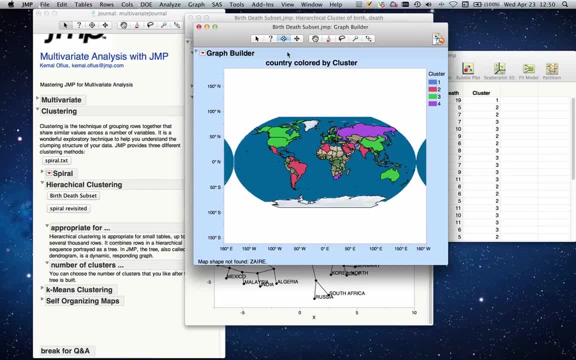 it on my. once I copied on my clipboard I can paste it in my PowerPoint or Word document. So this is how we would approach to hierarchical clustering. and just to reiterate, hierarchy clustering is appropriate for small tables and you can choose the number of clusters once you build the tree. Second item in our 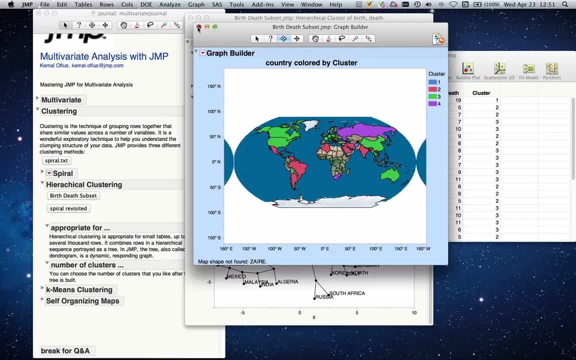 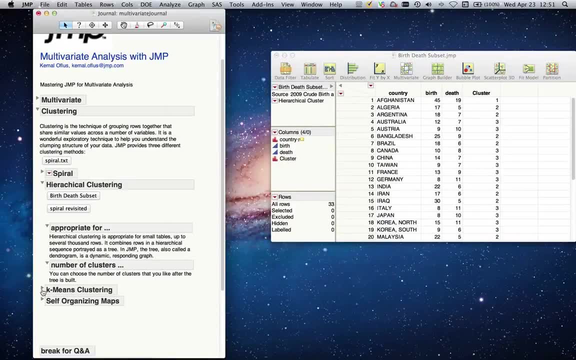 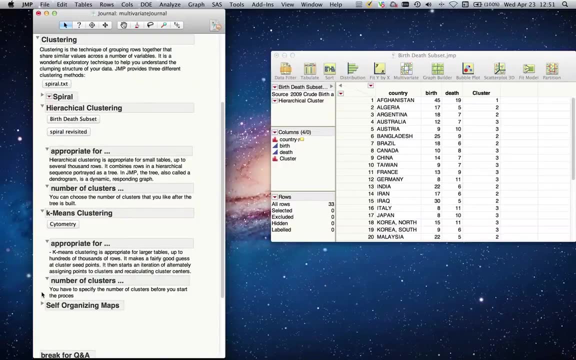 list of clustering is key-means clustering and before I go there, let me close these windows so we will have more real estate to work with. Key-means clustering is appropriate for larger tables and you have up to hundreds of thousands of rows and this makes it a fairly good guess at cluster. 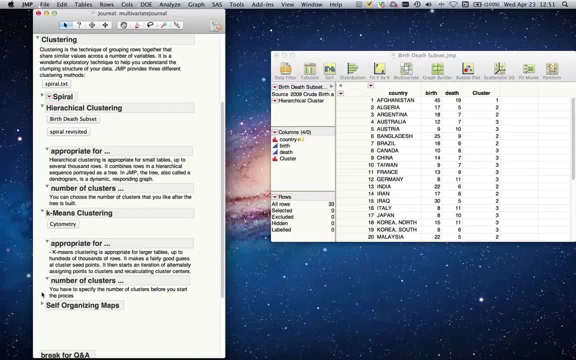 seed points It starts with. it'll start with the guess of what the center seed points are and then it iteratively assigns points to these clusters and recalculate the cluster centers. and the difference between hierarchical clustering and key-means clustering is that you have to specify the number of clusters before you start the process. 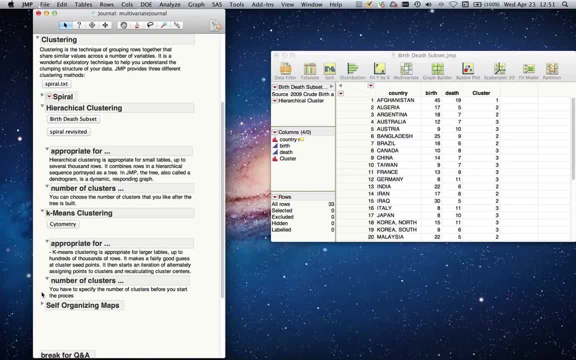 And that makes sense, because if I say I want three clusters, it will assign three center points to my cluster seeds and then iteratively go through each of these observations to assign them to more appropriate clusters. And let's look at this as an example. again, I have the data set for cytometry. 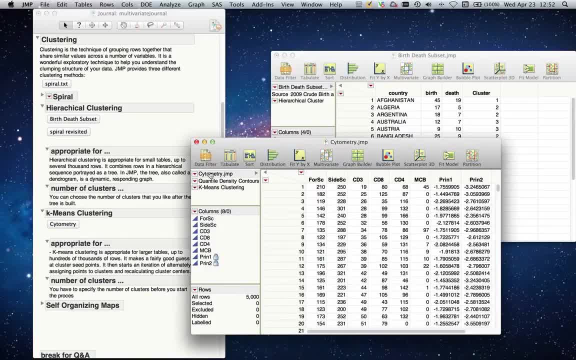 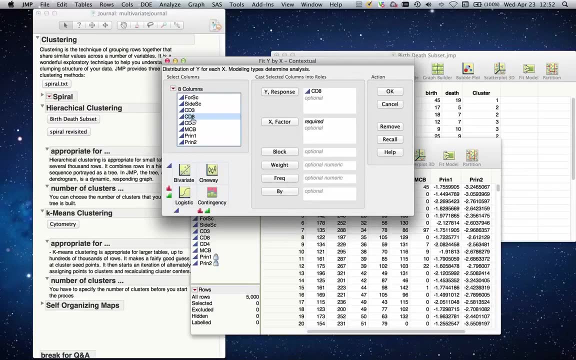 It's the cytometry readings. And if I just look at the data, let's look at the data for a second. If I want to see the difference between, let's just see if there's any kind of correlation. I'm trying to fit my CD8 data, for example, to my CD4 data. 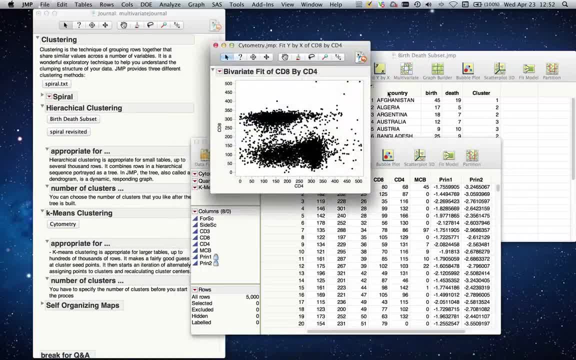 And if I see if there's any kind of relationship, it's like individual and I can see there are two separate groups. But I want to be able to specify this with other variables as well. So let's look at our clustering methods, see how they will perform. 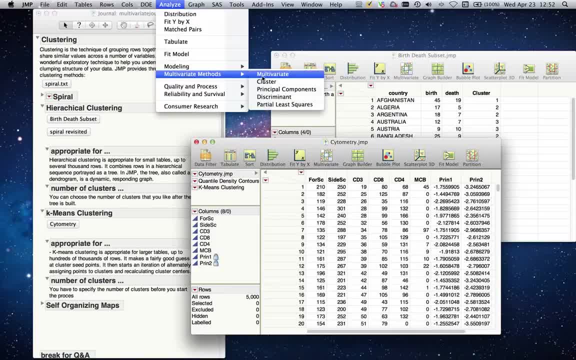 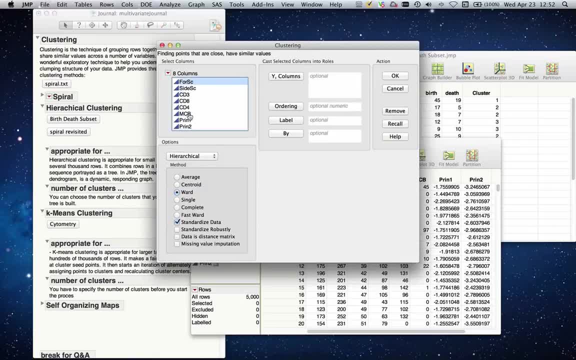 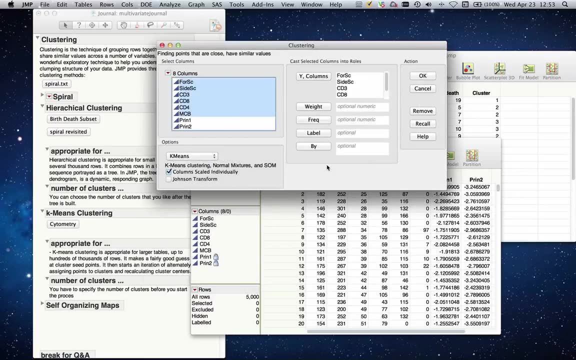 Under Analyze Multivariate Methods- Cluster, And I will select all my variables put into my Y columns Instead of Hierarchical. now I will select K-Means- Clustering And I will leave the default options on And I will not go into any more details here. 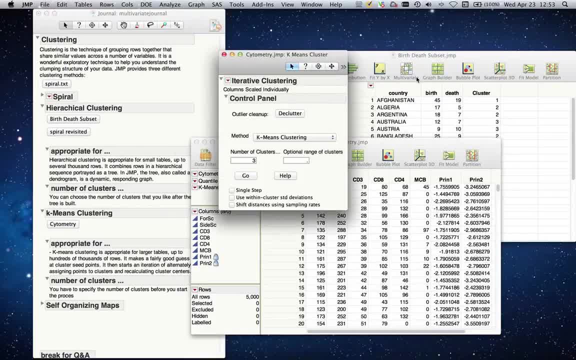 And say OK. What will happen is it will give me the iterative clustering platform, And this is where you will also find self-organizing map, which we will cover next. Let's leave it as K-Means. Clustering And declutter option will give you choice to clean out outliers, basically. 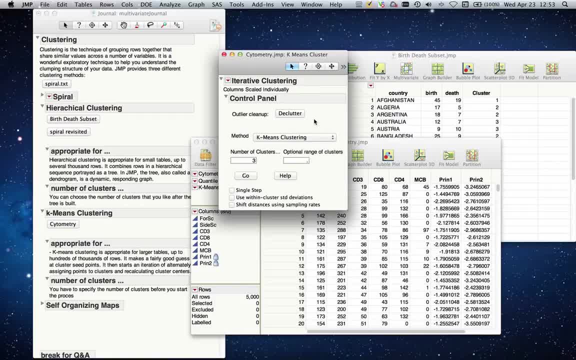 Declutter your dataset, so you will be focusing on the more general explanation of your data. Again, just to keep in mind, clustering is an exploratory data analysis, Not necessarily predicting, But once you create these clusters, you can use them as a predictive column as well. 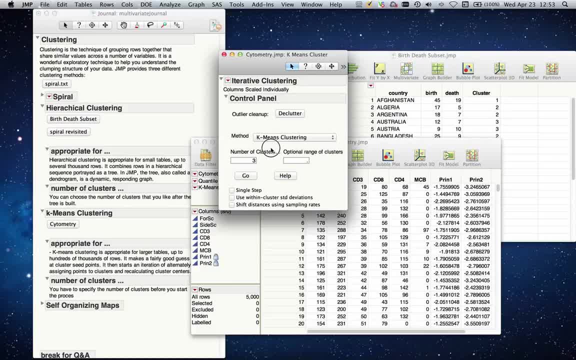 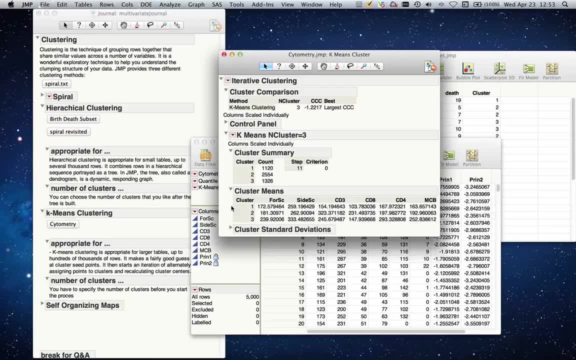 So I will select my number of columns as being 3. And I will say Go. What will happen now? is it built 3 separate clusters for me And put them into separate groups And says I have 1100 for cluster 1,, 2500 for cluster 2,, 1300 for cluster 3.. 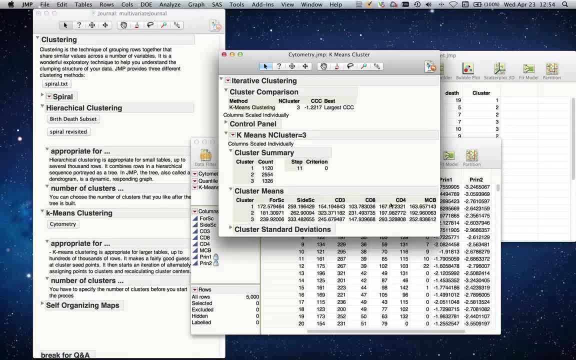 And also gives me the means for each of these variables, where each of these clusters fit. And, like I did earlier, once you build a cluster you can do a biplot And you can see how each of these clusters fit on my dataset. 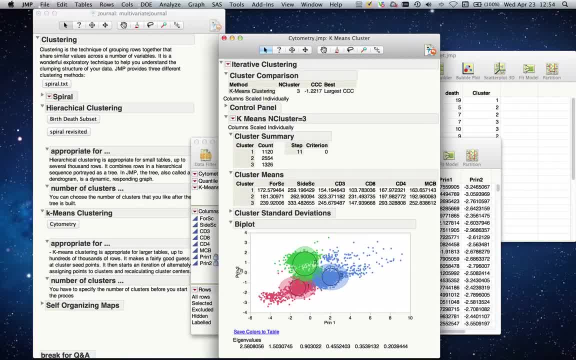 And what you notice here is that it uses the principal components Which we will be covering in the next section of this WebEx. In principal components, we were trying to take all these variables And make them as descriptive as possible And create two principal components. 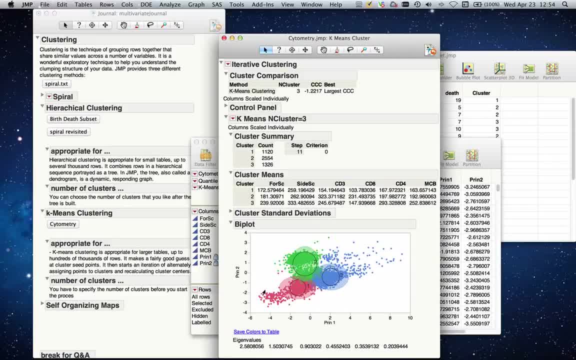 You can have as many principal components as you are comfortable with, But this biplot we are looking at first two, And then you can see the concentration of these data points in different clusters And, like I talked about earlier, you can save your clusters to your data table. 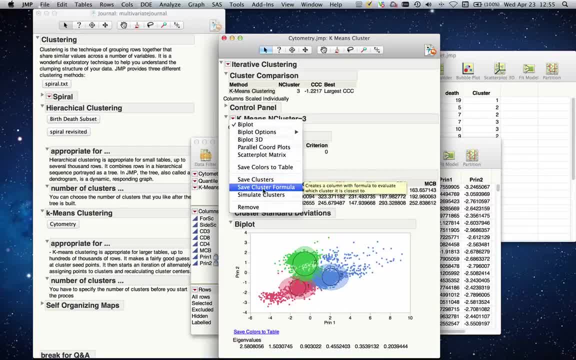 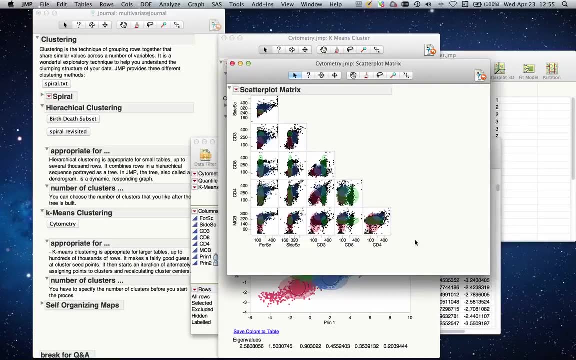 You can save a formula that creates these clusters That you might want to use later on in another dataset To see if your clusters will hold. And just another thing to look at here is the scatterplot matrix And you can see each of these variables and how they relate to each other. 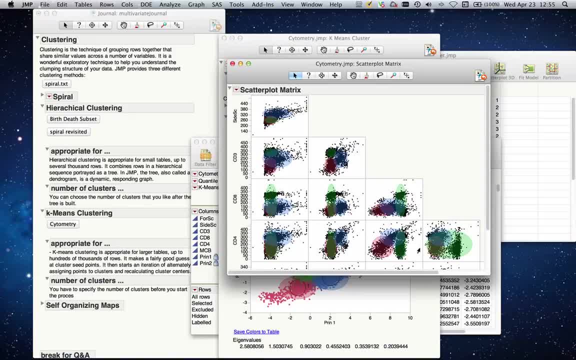 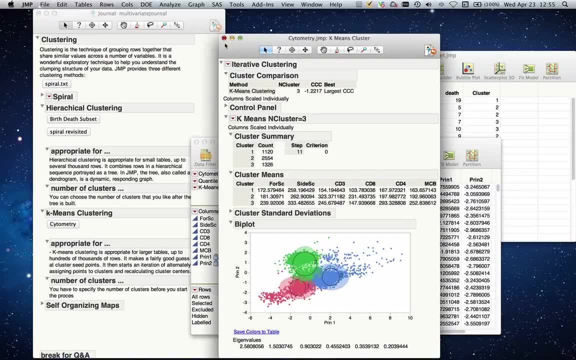 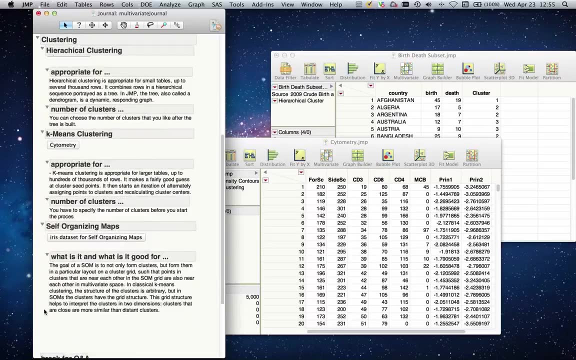 With different clusters. This is another way of looking at it. And let me close this And the next topic I would like to cover here is the self-organizing maps, And again we will follow the same idea that we talked about. 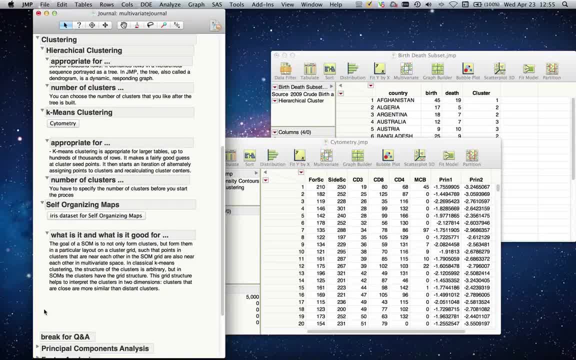 With the hierarchical clustering, and k-means clustering. What is it good for? What is it that much good for? Self-organizing maps are not only to form clusters, But also to form them in a particular layout in this grid, So that the points in the clusters are near to each other. 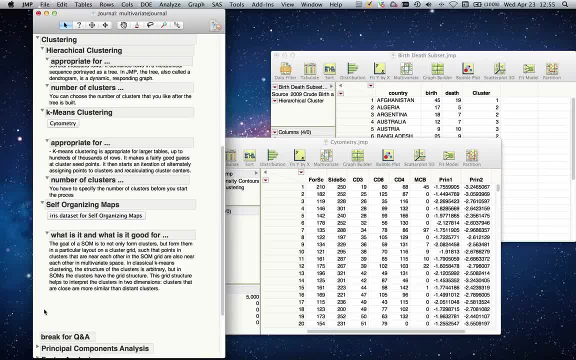 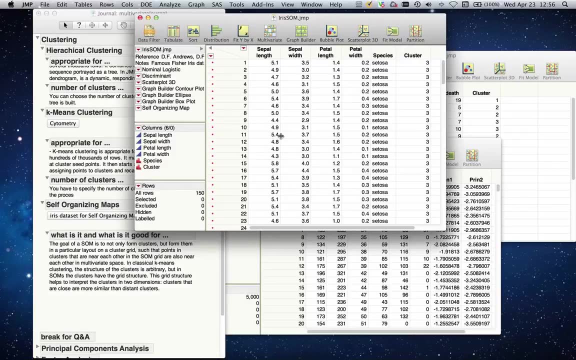 As if it's a map In this multivariate space. So let's look at the example And then maybe it will become clearer in that sense. I have this iris dataset. It's a very famous dataset. It's been used a lot on exploratory data analysis. 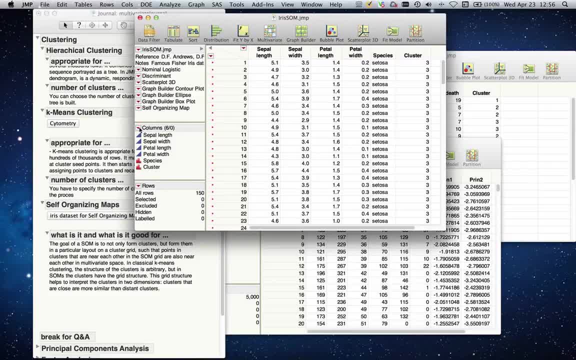 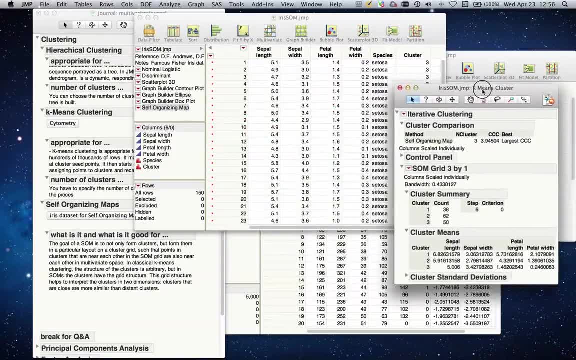 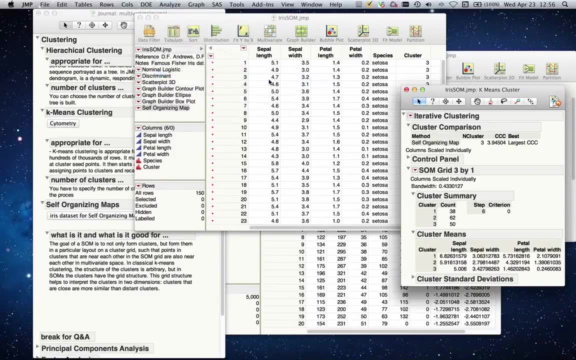 Especially in the multivariate world. So let me show you what the output looks like. first, It's a self-organizing map. Let's put this aside Under analyze Multivariate methods- Cluster, And I will select all the variables that I have. 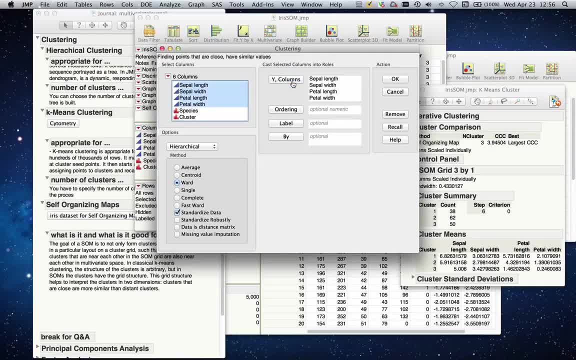 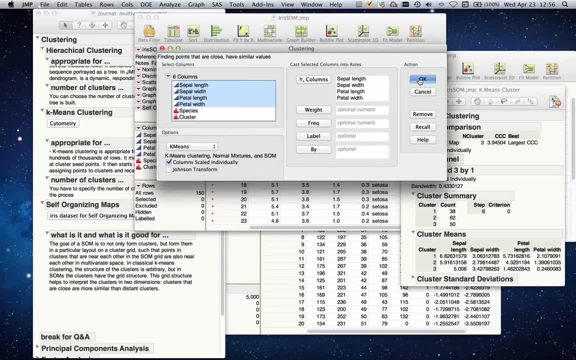 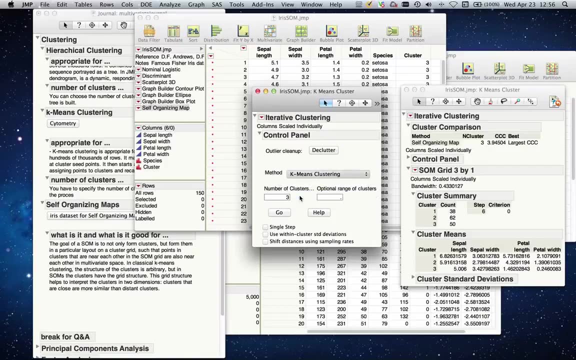 Since I don't know which one will be more descriptive, Put into my columns. Under the options, I will select k-means And say OK In the k-means platform. now I can select my method to be self-organizing map. 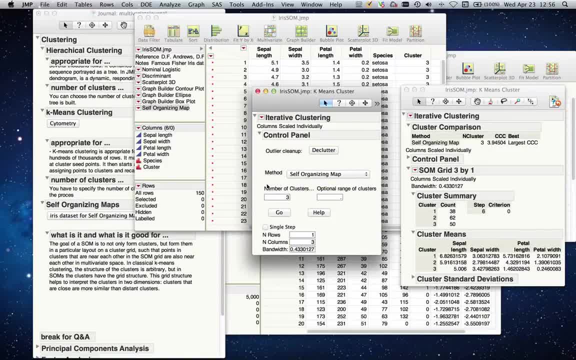 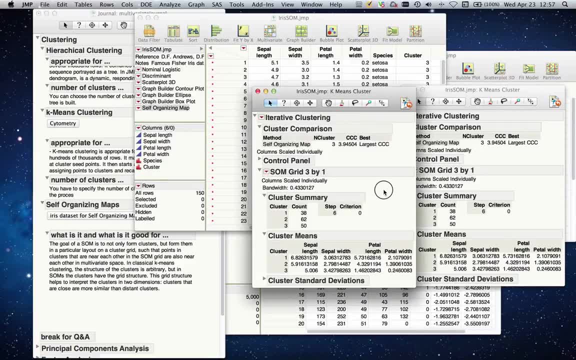 And you can change the number of clusters to whatever, However many, you're comfortable with, And then I will say go. What will happen is Again: organize my data into three separate clusters Where there are 38 observations for cluster 1.. 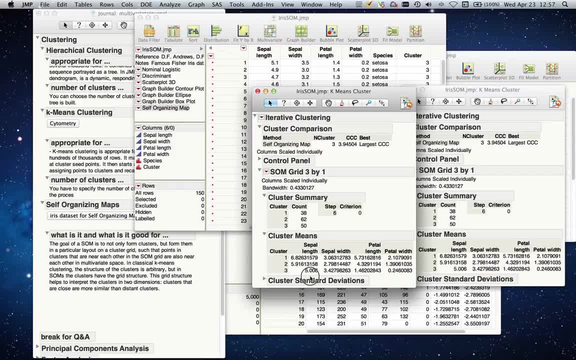 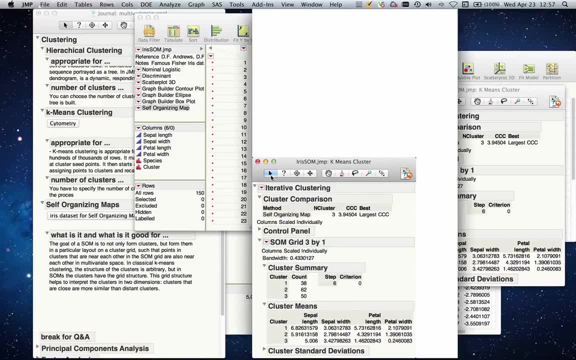 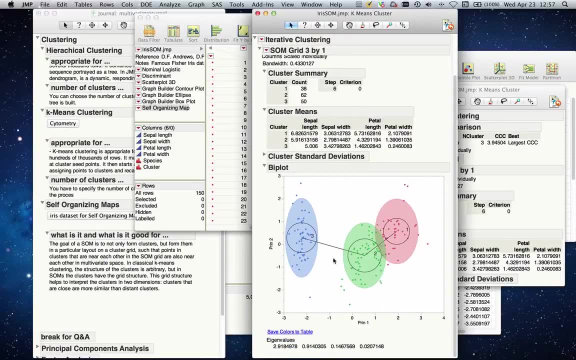 62 for cluster 2. And also collected the means for each of these clusters And I can come back and look at my biplot now And I can see, If you remember, In the k-means clustering They were kind of close to each other. 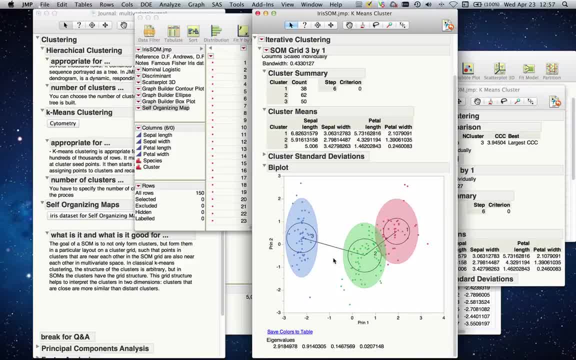 But way off from each other In some sense. In the self-organizing map You will see, as if this is a map, These clusters are very close to each other Geographically in the principal components: space. Now let's go back to what we started with in our data set. 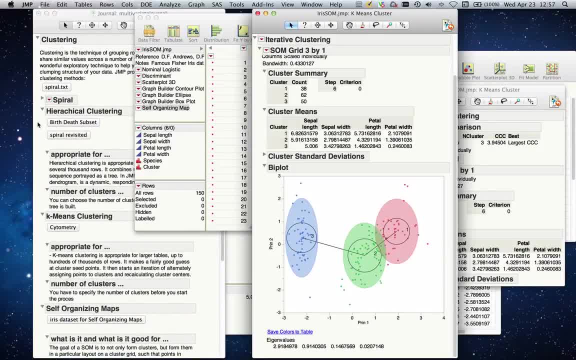 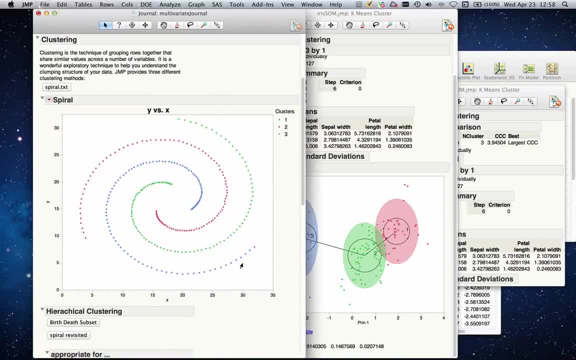 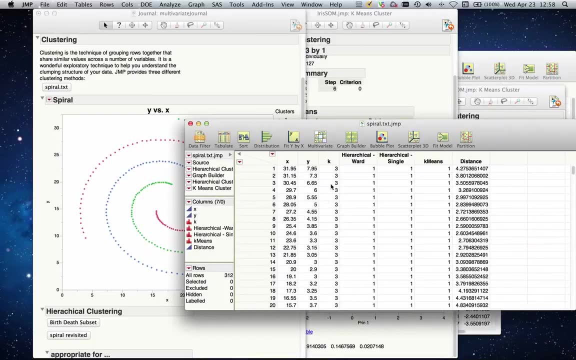 We had a spiral And we were trying to identify Which clusters of each of these colors Fit into. So let me open my data set- Spiral data set- And I went through all these analysis And I built different Clustering algorithms to identify which one will be more useful. 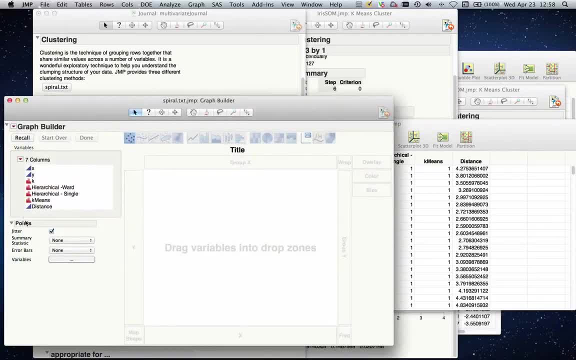 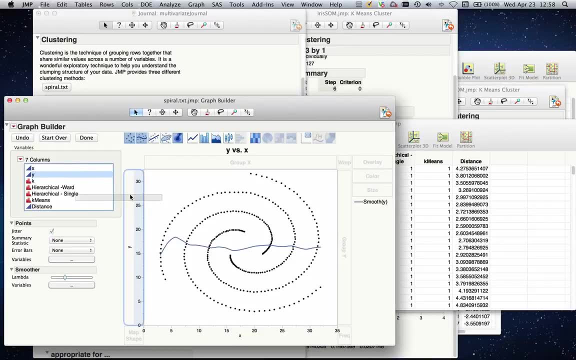 Let's go to my graph builder And then look at the picture. I have my X coordinate, Y coordinate. It's my old data set. They're all in black. Now I want to color it by. Let's start with the k-means clustering. 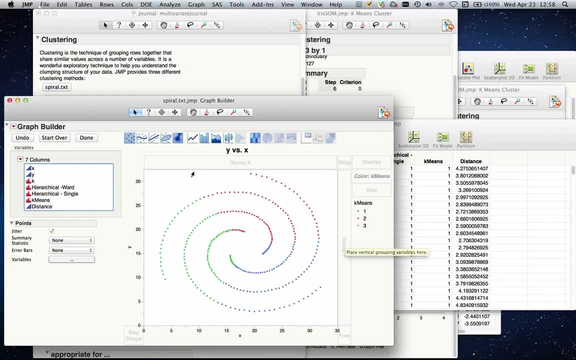 And see what it looks like. So I can see visually That k-means clustering divided my data into three separate groups And I can see here 120 degrees on each direction. So it took my space And divided into three separate groups.